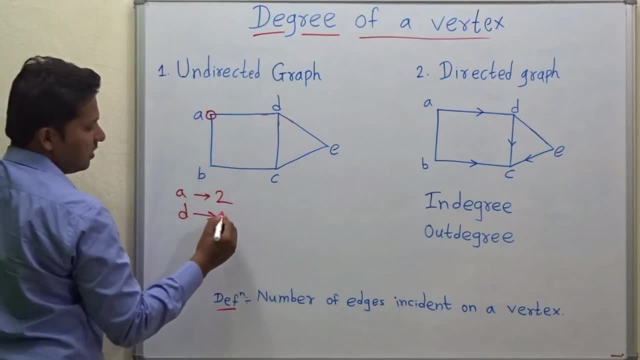 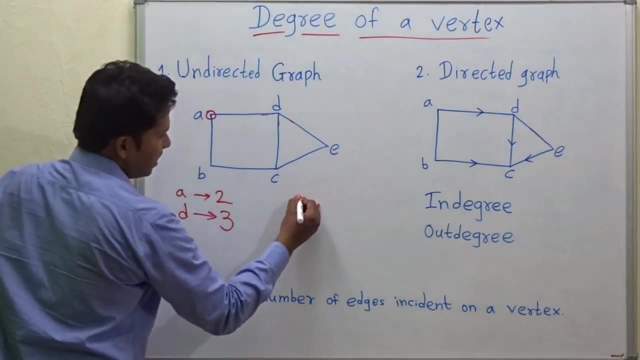 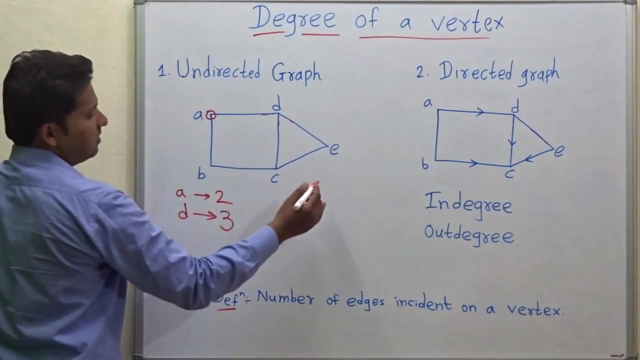 D, See 1,, 2 and 3.. So the degree of vertex D is 3.. Suppose, if there is a vertex for which there is no edge connected, okay, if the vertex name is N and there is nothing connected to this. 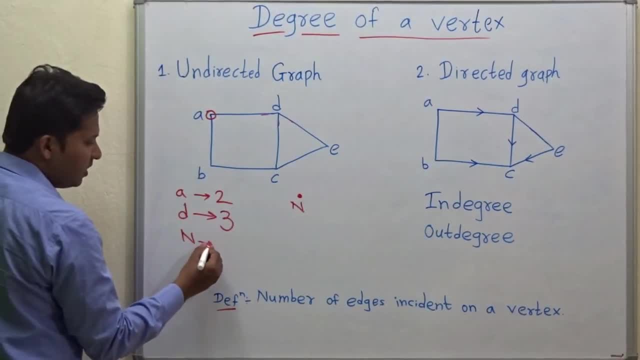 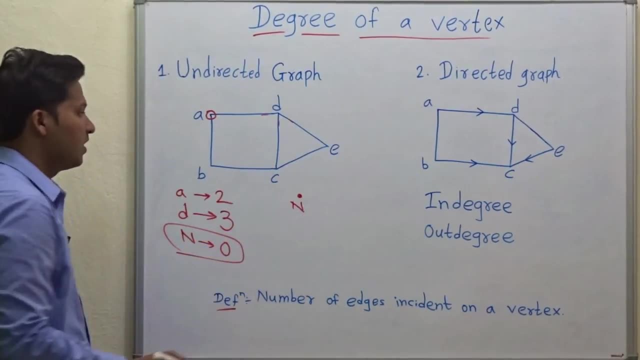 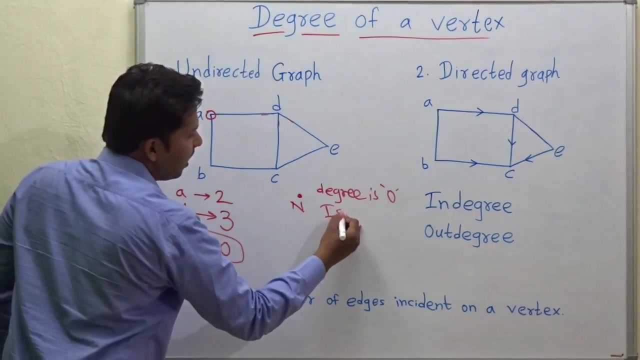 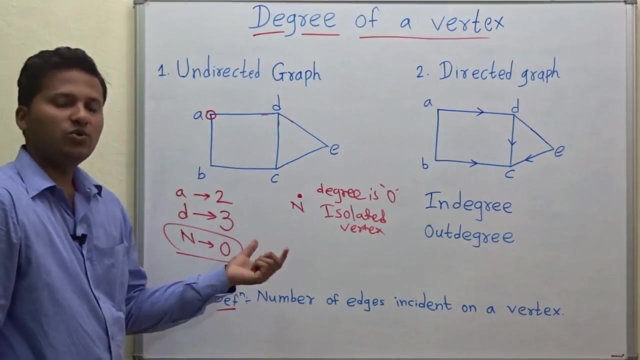 vertex, then degree of vertex N will be 0,. okay, So the vertex which is not connected to any edge means the degree of that vertex is 0, then that vertex is called as isolated vertex. Okay, this is called as isolated vertex. Now let us see an example of loops. What in case of? 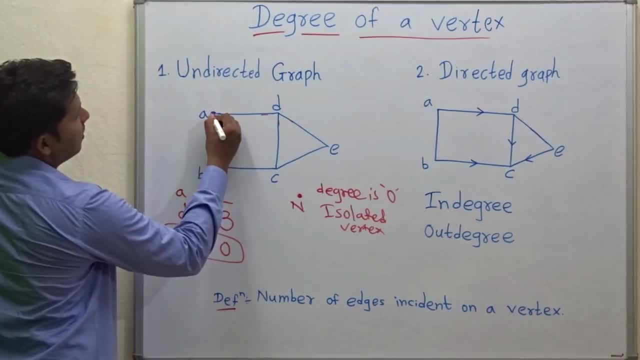 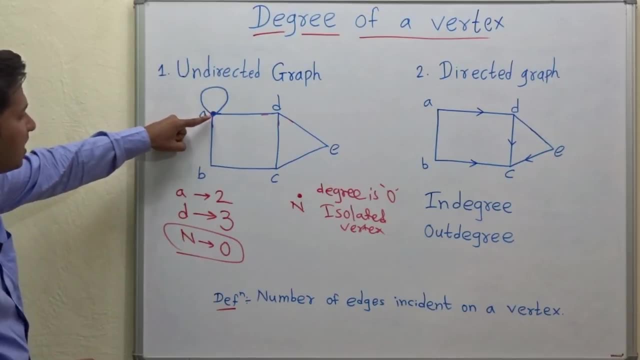 loops. So see, if this is the node, and there is a loop at, this node means there is an edge for which the starting point is A and end point is also A. okay, So this is a loop edge. This is the loop edge. 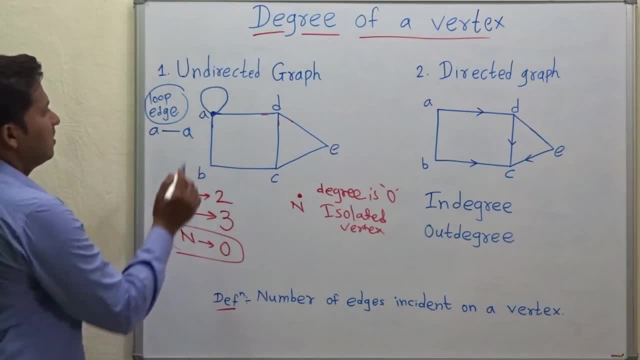 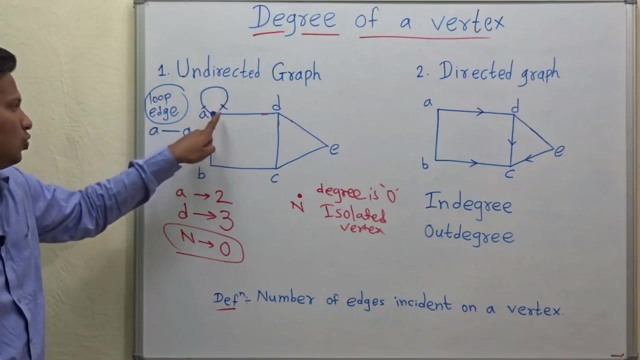 okay, So for loop edge, see, this is one edge incident and this is the second edge, right. So the degree for this loop edge is considered as 2, right? See, this is 1 and this is 2.. So two edges incident on. 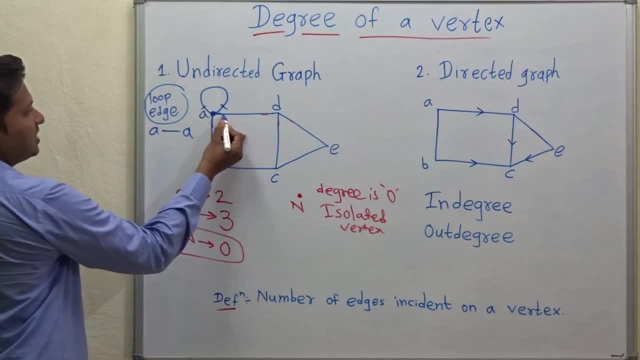 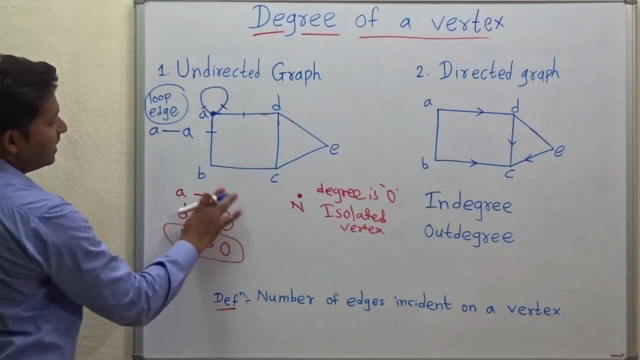 A, So degree is considered as 2, and other two edges are this edge and this edge. So the total degree for vertex A now is 4.. See, this is 1 edge, this is 2 edge, this is third and this is fourth right. So for a loop, 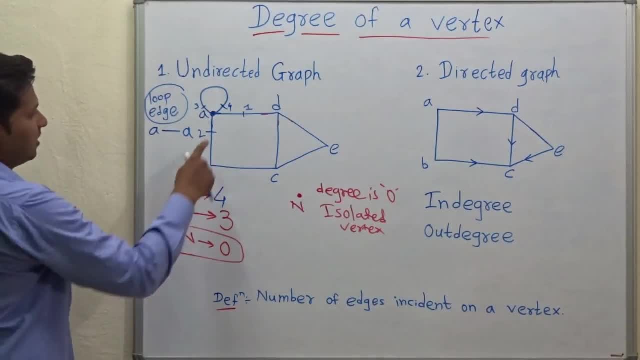 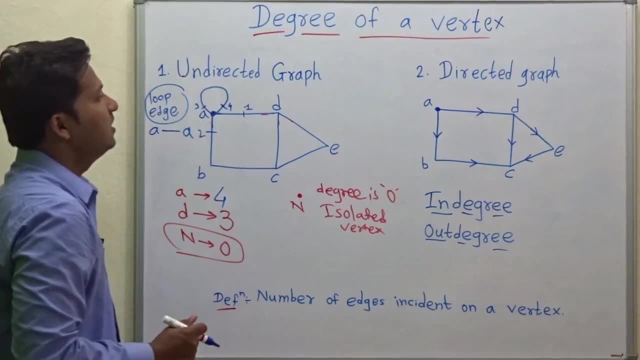 degree 2 is added to that vertex. So the degree of vertex A is 4 now. Now let us go to directed graphs. okay, So this was for undirected graph. Now we will see directed graph in which every 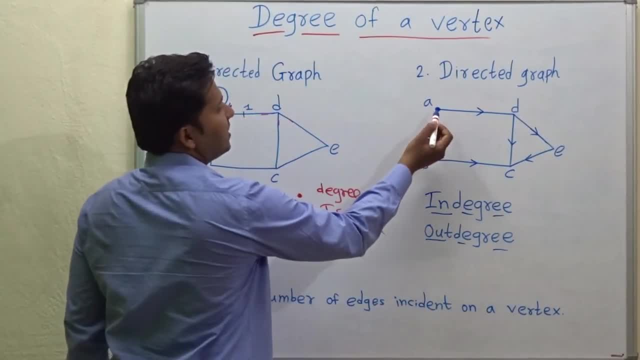 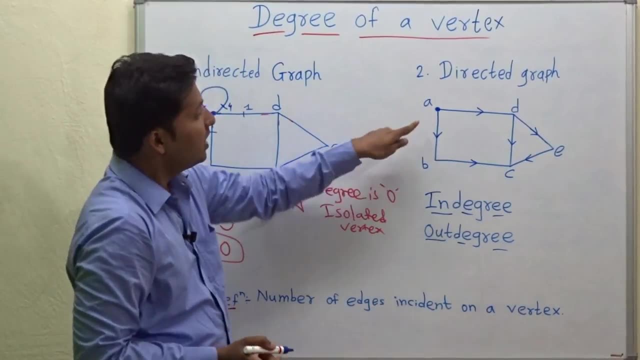 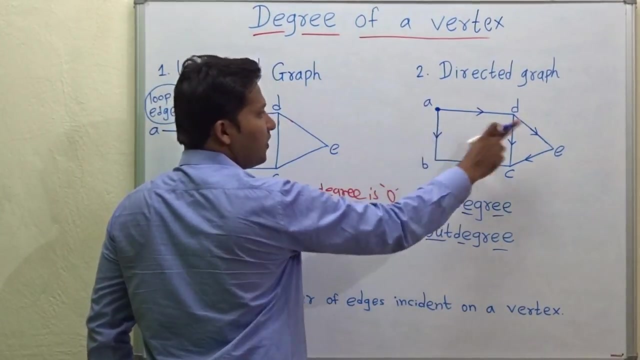 edge is directed. So now see what is the degree for A. See, here there are 2 edges connected to A, but these 2 edges go away from A, So this is A and these 2 edges go away from A, So this comes in out degree. Okay, see for degree. 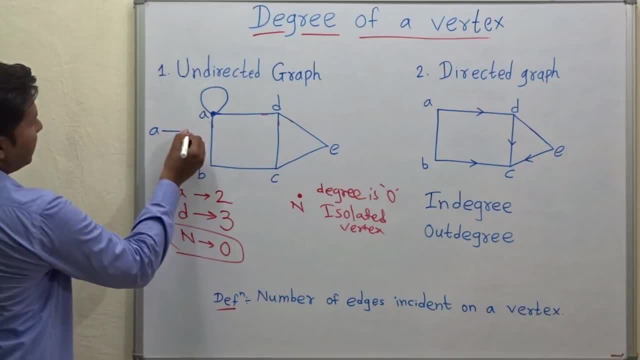 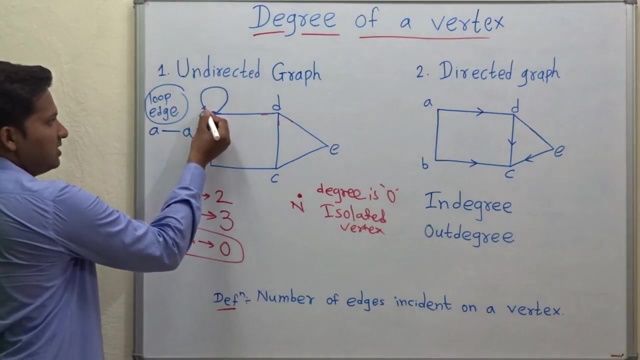 which the starting point is A and end point is also A. okay, So this is a loop edge, This is the loop edge. Okay, So for loop edge. see, this is one edge incident and this is the second edge. right, So the? 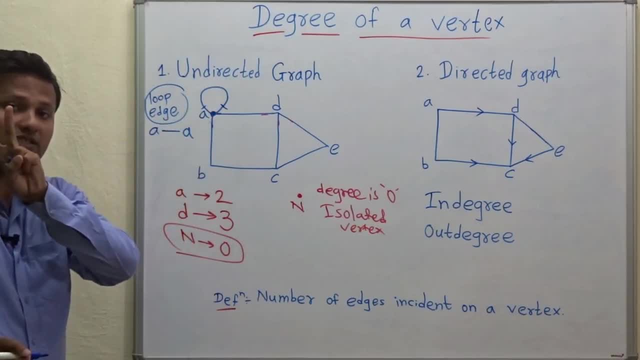 degree for this loop edge is considered as 2, right See, this is 1 and this is 2.. So two edges incident on A, So degree is considered as 2.. And other two edges are this edge and this edge. So 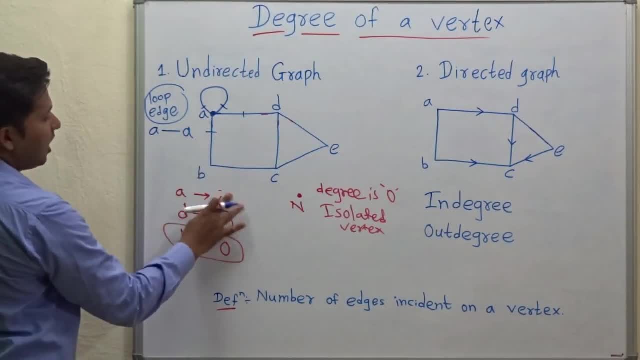 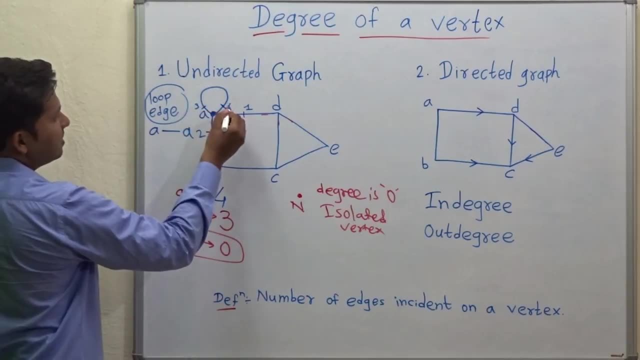 the total degree for vertex A now is 4.. See, this is 1 edge, this is 2 edge, this is third and this is fourth right. So for a loop, degree 2 is added to that vertex. So the degree of vertex A is 4 now. Now let us go to. 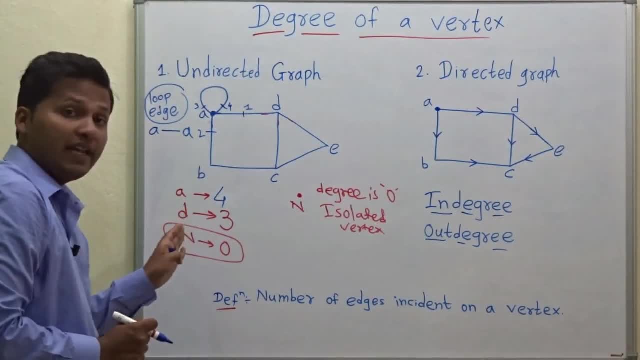 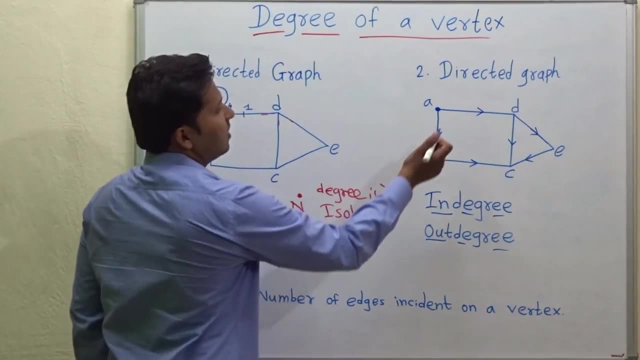 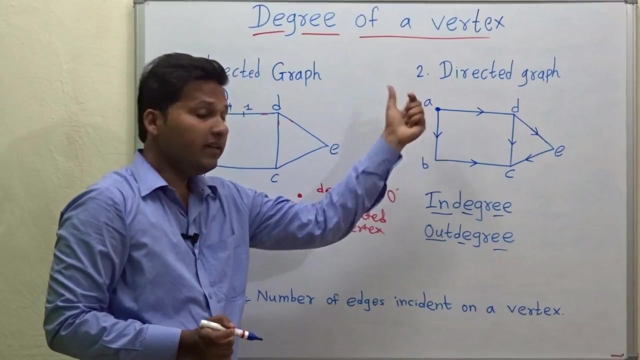 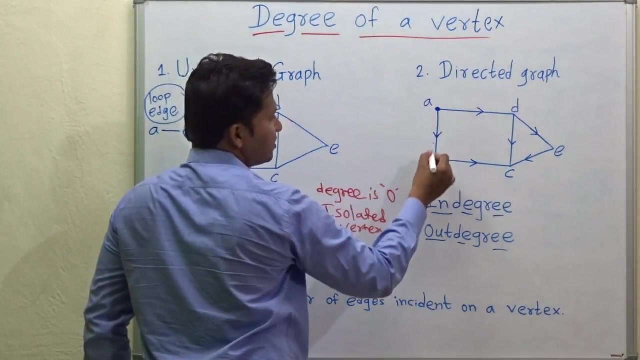 directed graphs. okay, So this was for undirected graph. Now we will see directed graph in which every edge is directed. So now see what is the degree for A. See, here there are two edges connected to A, but these two edges go away from A. So this is A and these two edges go away from. 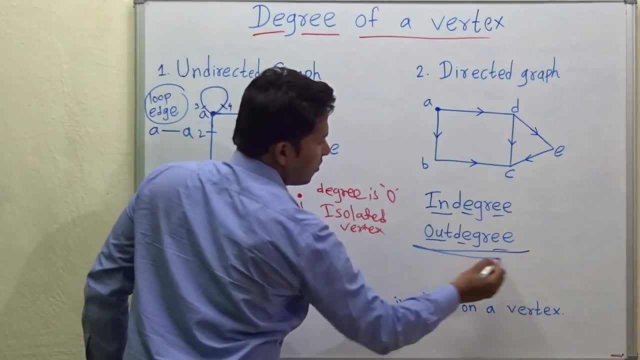 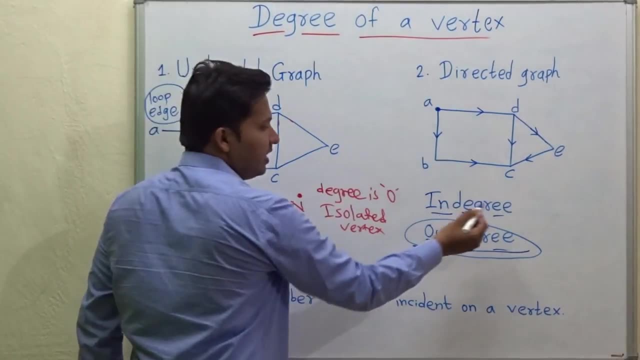 A, So this comes in out degree. okay, See for degree of edges in directed graph. there are two types in degree and in directed. So this is A and this is out degree. So this is A and this is. 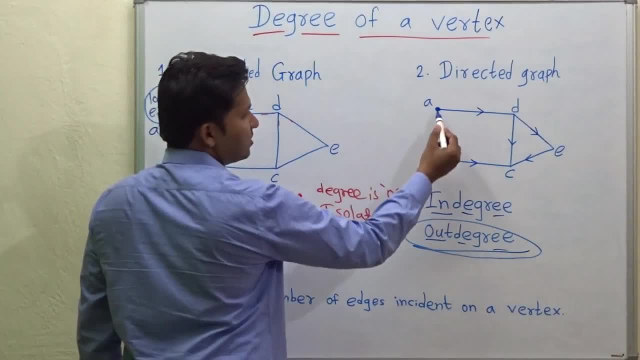 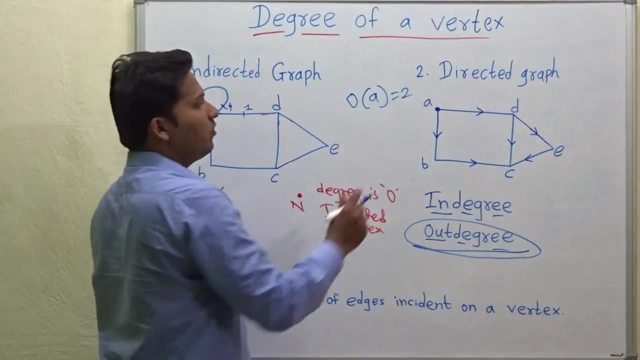 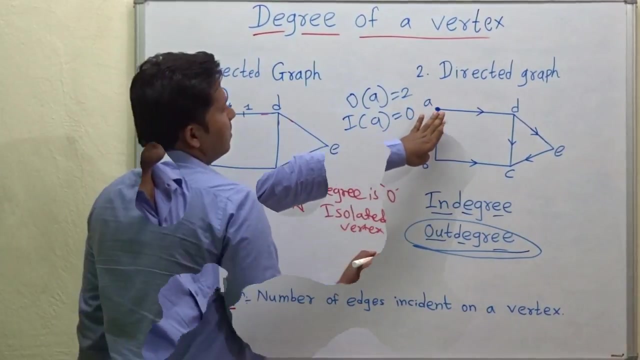 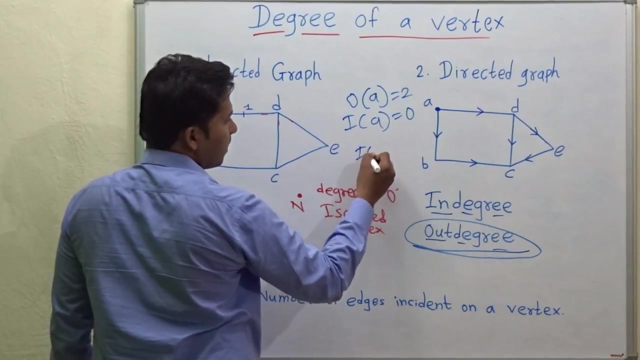 out degree. right, So these two edges going away comes in out degree, So out degree of A will be 2.. And what is the in degree of A? In degree of A is 0, because there is no edge coming towards A. Now let us see for vertex B. So for vertex B, in degree is 1 and out degree is 1.. 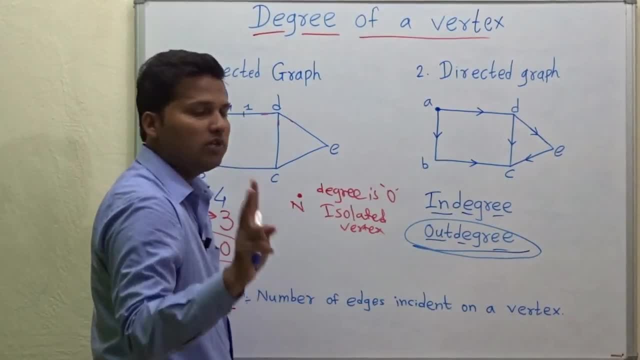 of edges in directed graph. there are 2 types in degree and out degree: right, So these 2 edges go in the from&prearth to&Degrees to&��ther grapes. there are 2 types in degree and out degrees: Right, so these 2 edges. 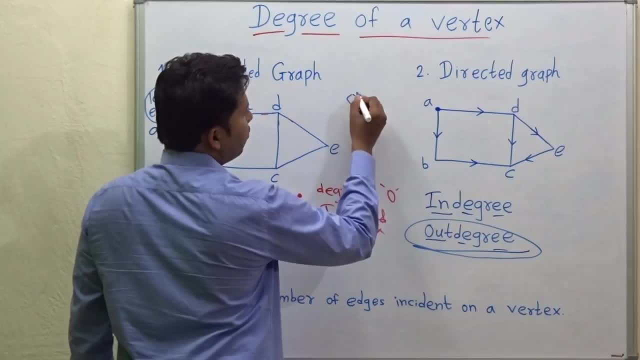 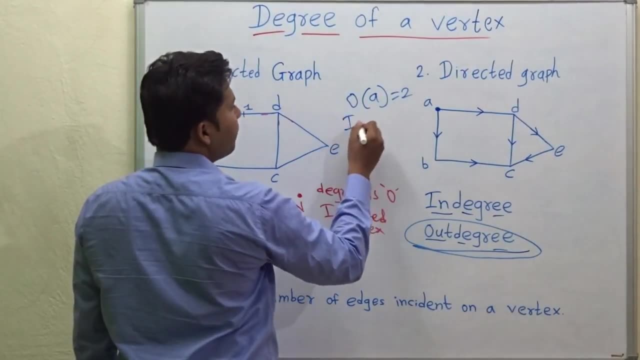 right. So these two edges going away comes in out degree. So out degree of A will be 2, and what is the in degree of A? In degree of A is 0, because there is no edge coming towards A. Now let us. 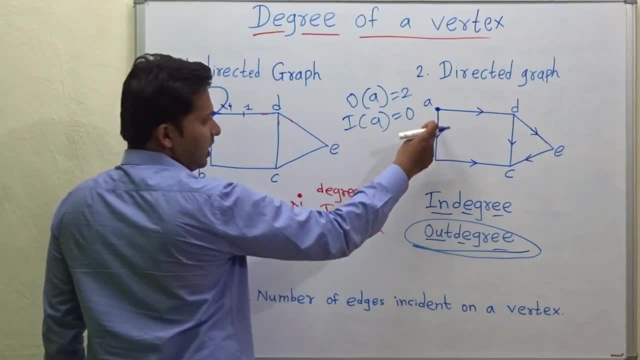 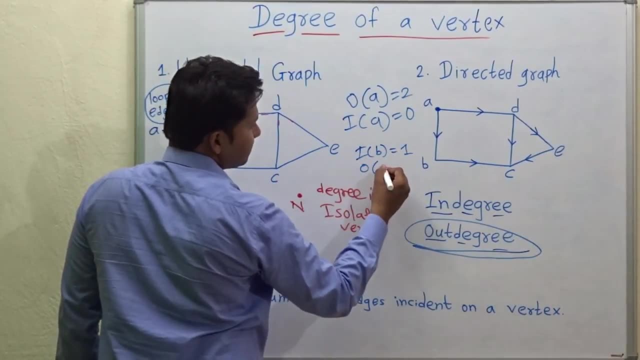 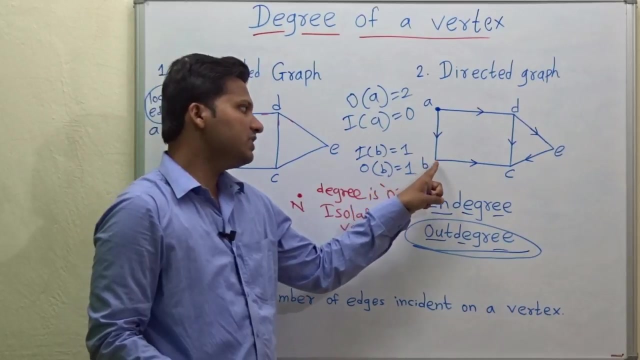 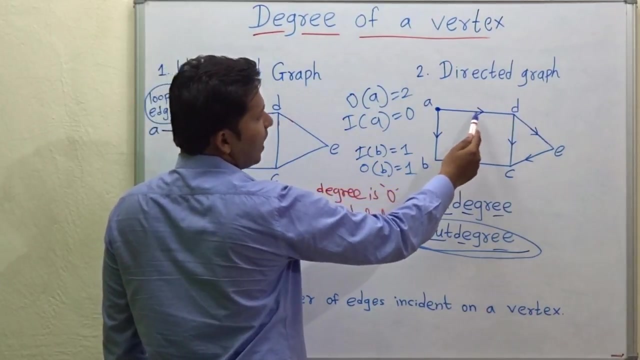 see for vertex B. So for vertex B, in degree is 1 and out degree is 1.. Right, Because there is one edge coming towards B and one edge going away from B. Right Now for vertex D, C in degree is 1,. 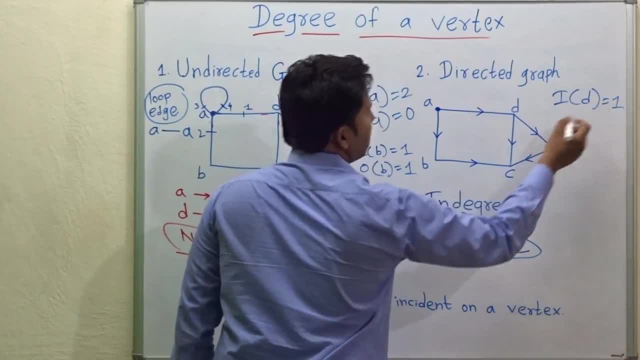 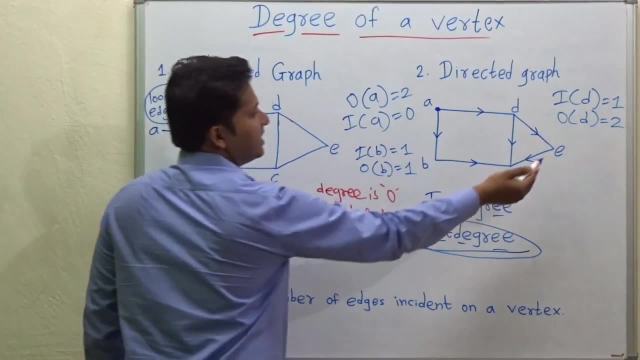 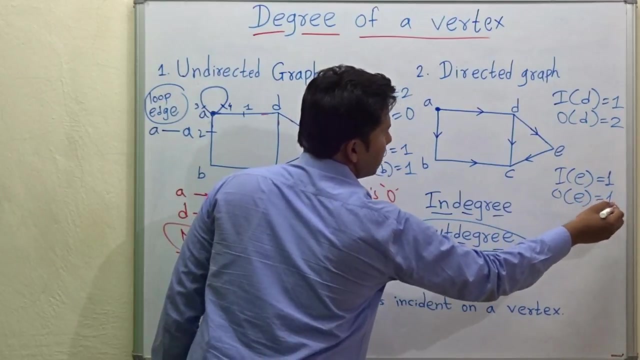 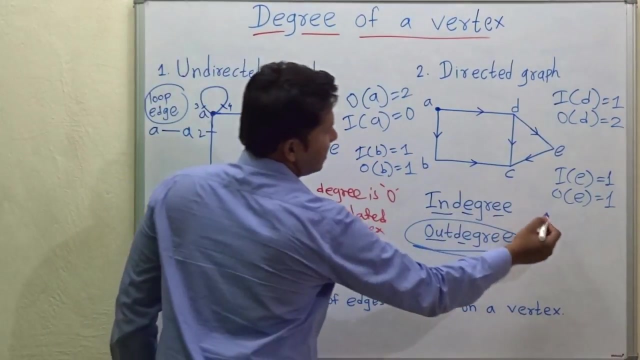 in degree for vertex D is 1 and and out degree is 2.. Then for vertex E: in degree of vertex E is 1 and out degree is 1, because one edge coming towards E and other edge going away from E. Now for vertex C. 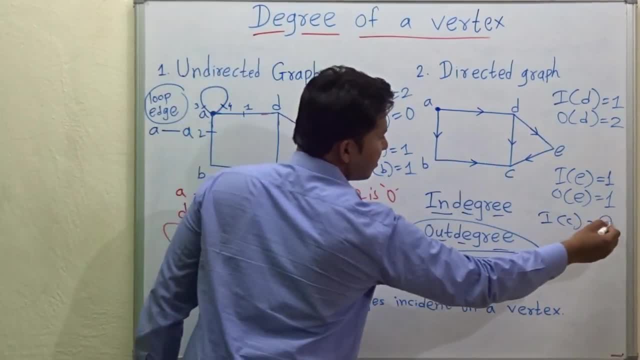 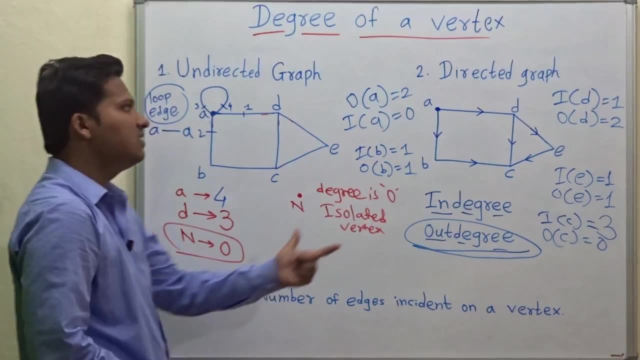 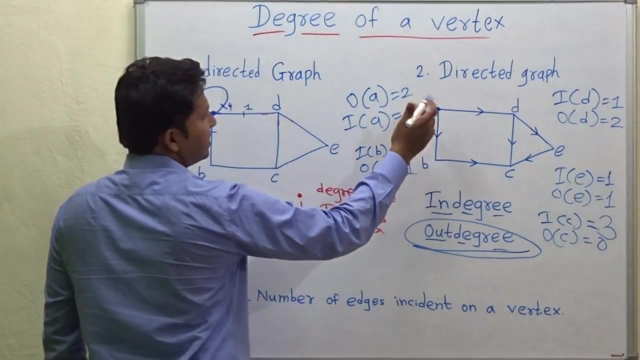 in degree will be 3, because all three edges are coming towards C, but out degree is 0.. Okay, so these are the in degrees and out degrees in case of directed graphs. Now let's see in case of loops. So if this is the vertex A and if here is a loop, okay, and this is the direction of the. 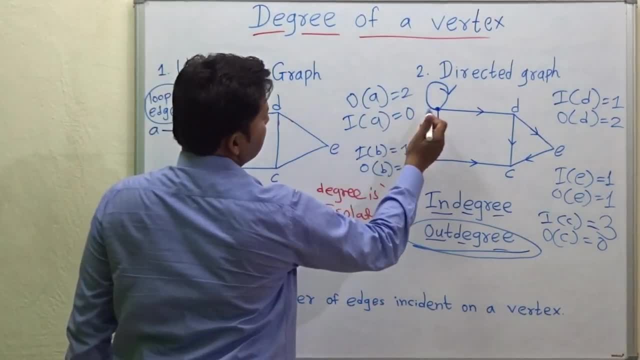 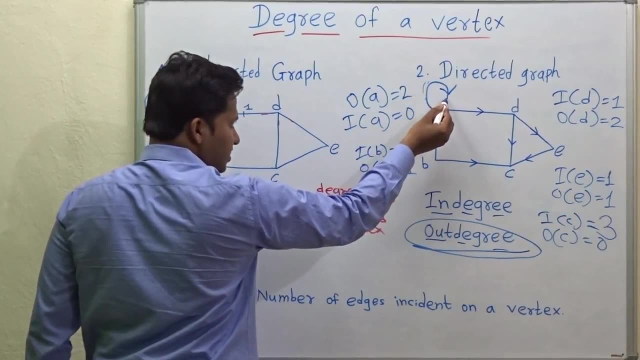 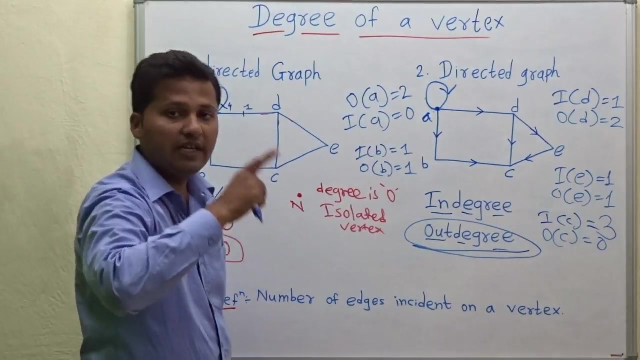 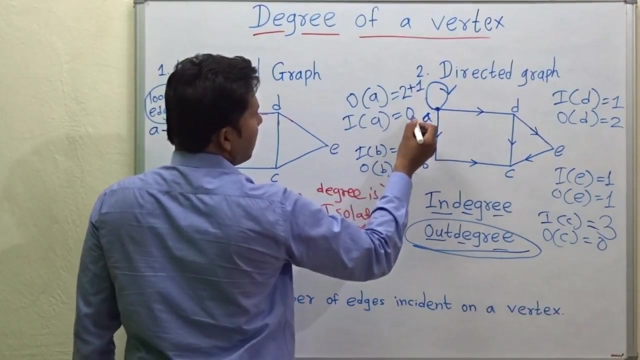 loop right. So this is very simple. See for vertex A. there is an edge going away from A and there is an edge coming towards A right. In this loop there is an edge coming towards A loop. So 1 is added to both in degree and out. degree means, see out, degree is 1, so plus 1 and 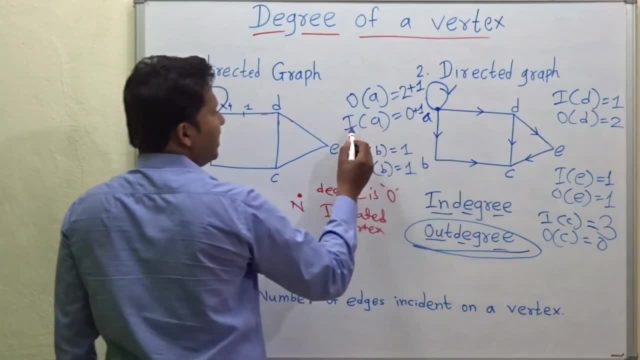 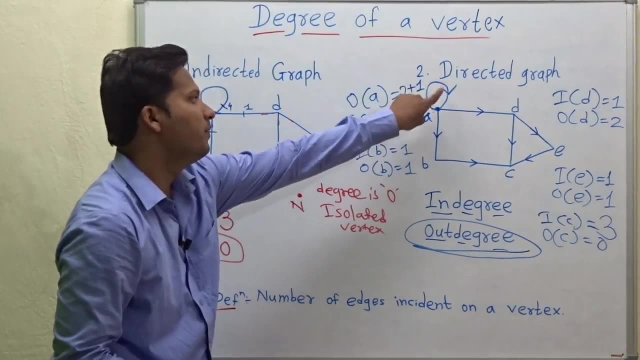 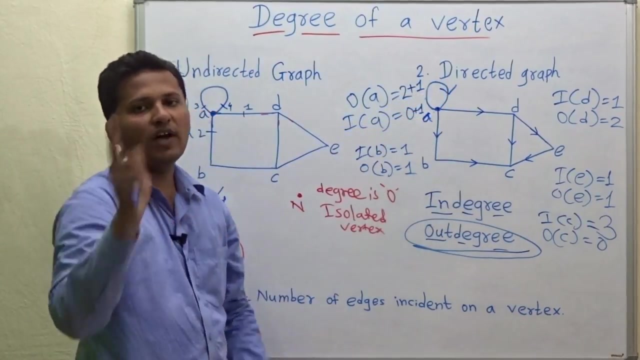 in degree is 1, so plus 1.. In degree of A will be plus 1 and out degree of A will be plus 1, because this is a loop and there is an edge going away from A and also coming towards A. So 1, 1 is. 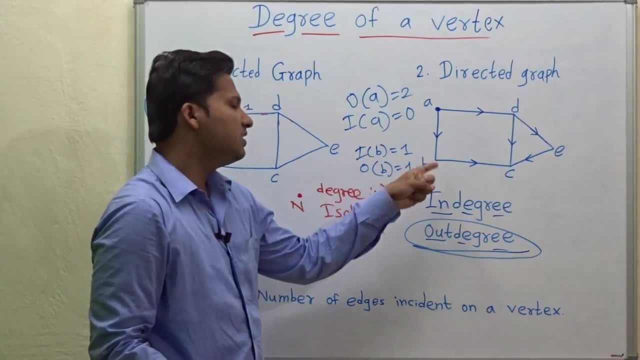 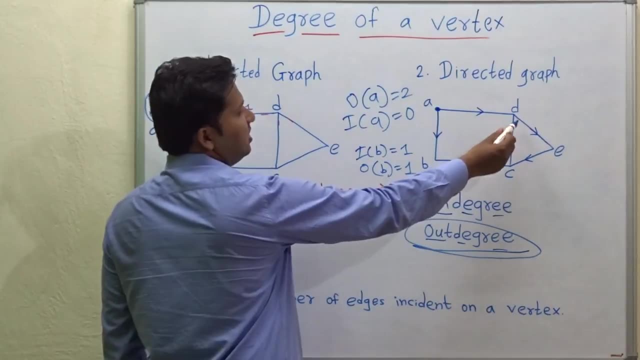 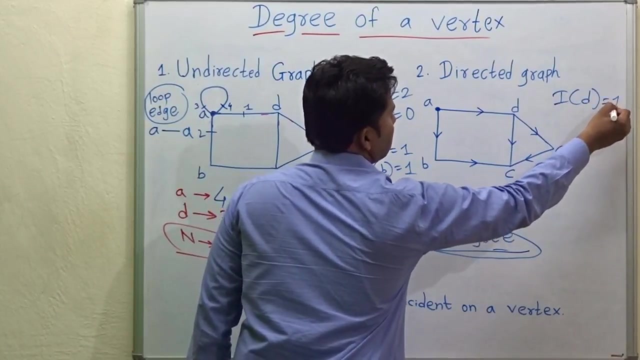 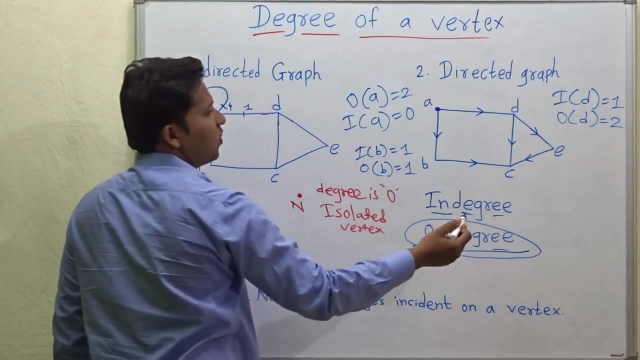 Right, Because there is one edge coming towards B and one edge going away from B. right Now, for vertex D, see in degree is 1, in degree for vertex D is 1 and out degree is 2.. Then for vertex E: in degree of vertex E is 1 and out degree is 2.. 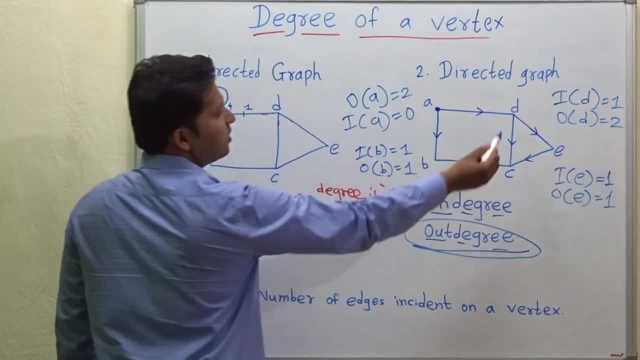 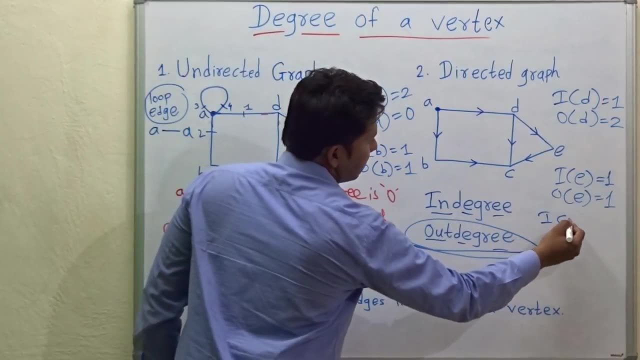 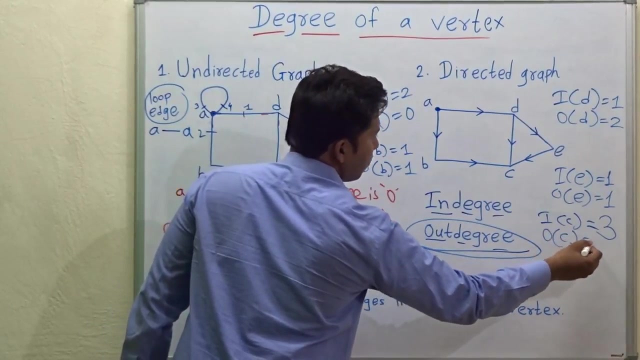 Then for vertex D, see, in degree is 1 because one edge coming towards E and other edge going away from E. Now for vertex C, in degree will be 3 because all three edges are coming towards C but out degree is 0, okay, So these are the in degrees and out degrees in case of directed graphs. 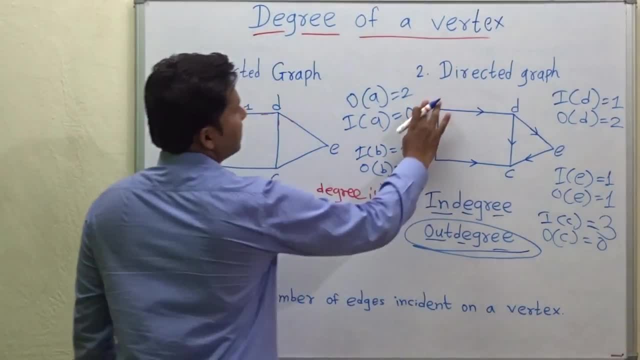 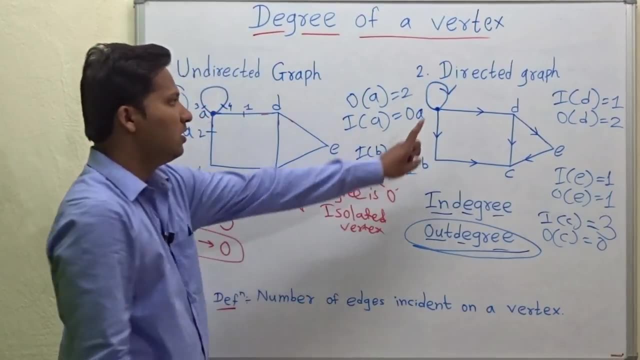 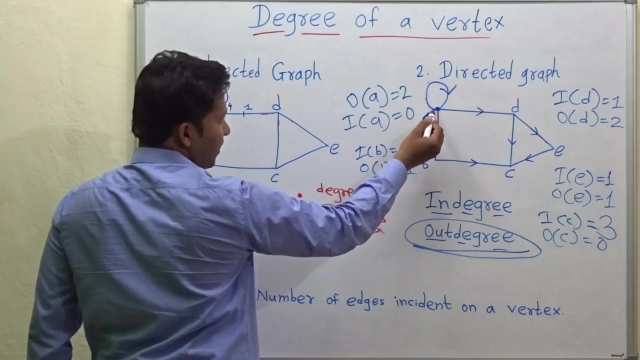 Now let us see in case of loops. So if this is the vertex A, if here is a loop, okay, And this is the direction of the loop, right. So this is very simple. See, for vertex A, there is an edge going away from A and there is an edge coming towards A. 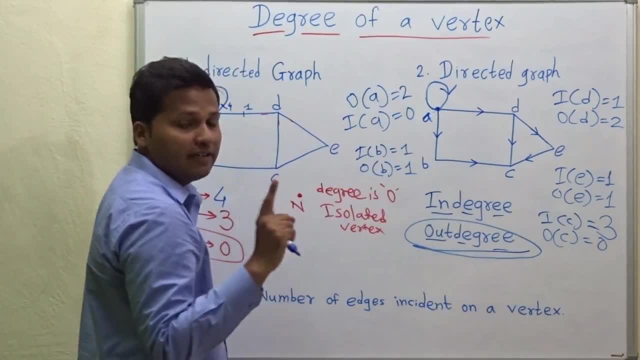 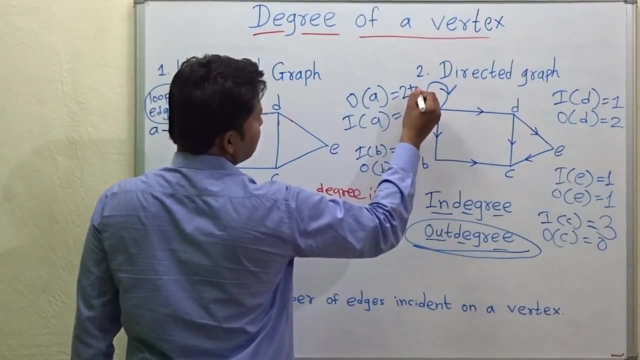 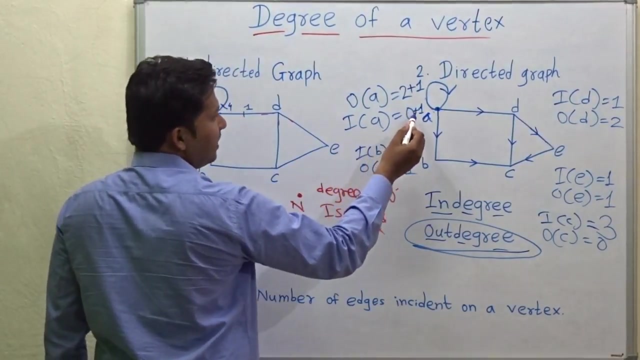 right In this loop. So one is added to both in degree and out. degree Means: see out degree is 1. So plus 1, and in degree is 1. So plus 1.. In degree of A will be plus 1 and out degree of A will be plus 1, because this is a loop. 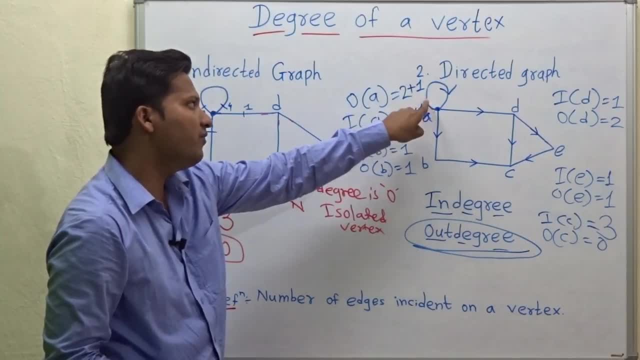 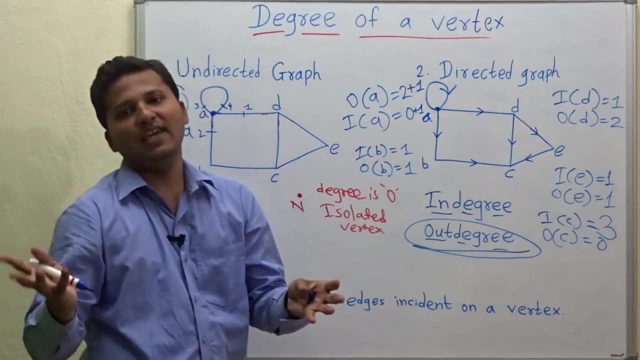 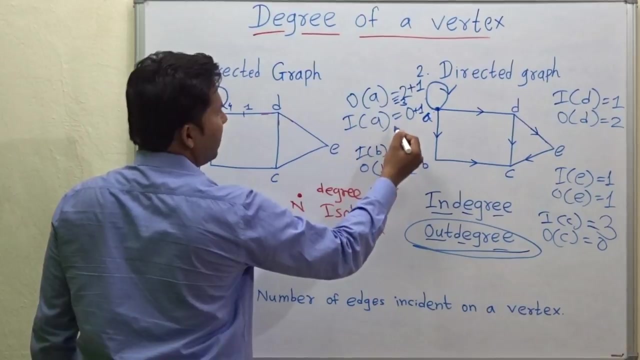 and there is an edge going away from A and also coming towards A. So 1, 1 is added to in degree and out degree of A. So this is in case of loops. So total out degree will be 3 for A and for in. 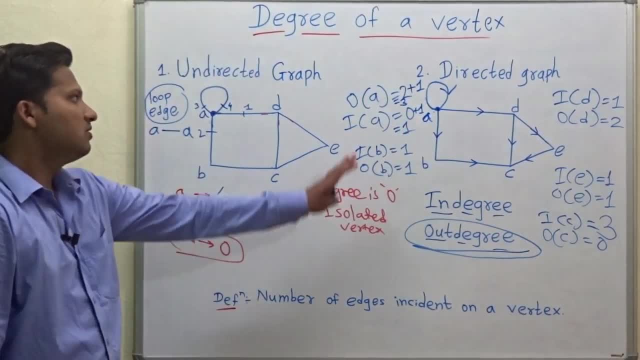 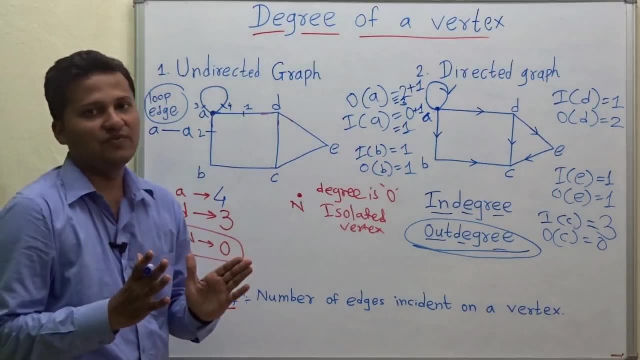 degree 0 plus 1 is 1.. So out degree is 3 and in degree is 1.. So this is the degree of a vertex in graph. Hey friends, please subscribe to my channel, as I post algorithm videos every day and if you. 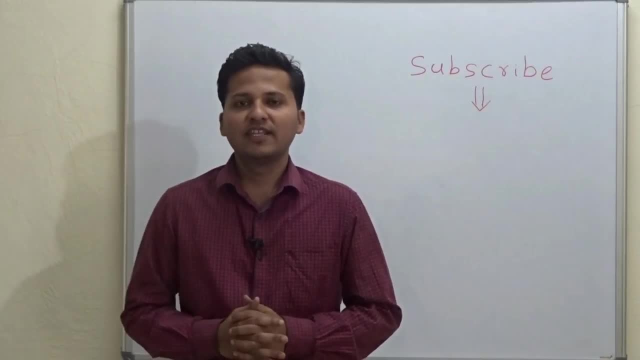 want a video on any particular topic, then please mention in the comment below. Thank you, 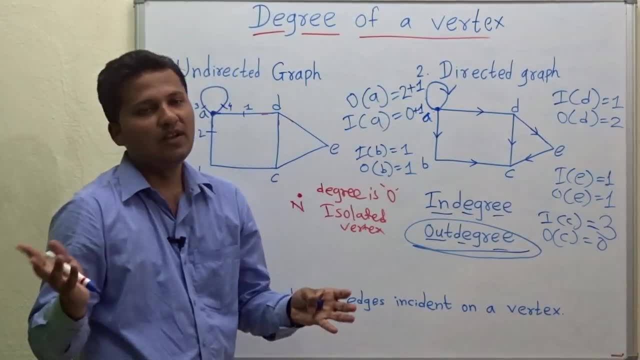 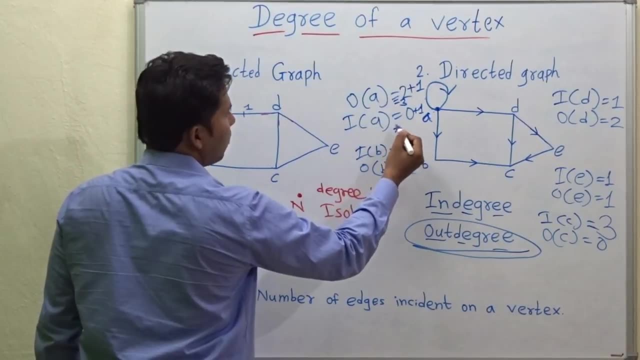 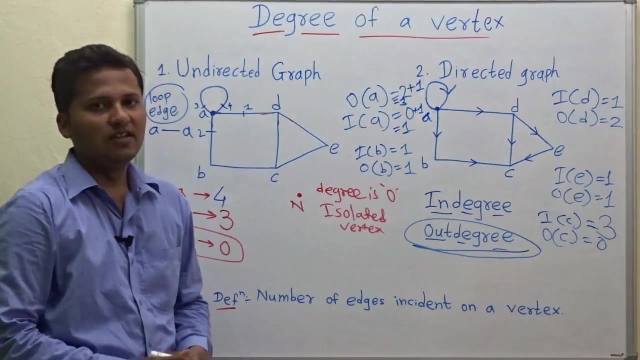 added to in degree and out degree of A. So this is in case of loops. So total out degree will be 3 for A and for in degree 0 plus 1 is 1.. So out degree is 3 and in degree is 1.. So this is the. 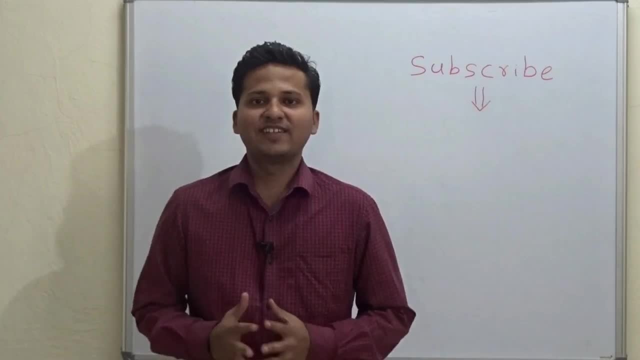 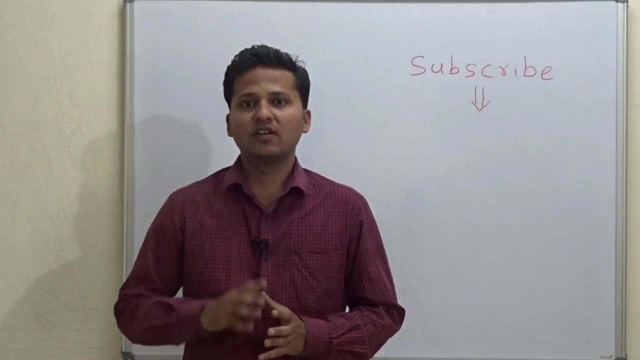 degree of a vertex in graph. Hey friends, please subscribe to my channel, as I post algorithm videos every day, and if you want a video of any particular topic, then please mention in the comment below. Thank you. 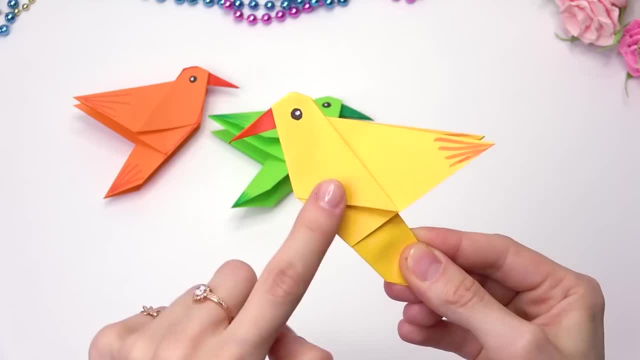 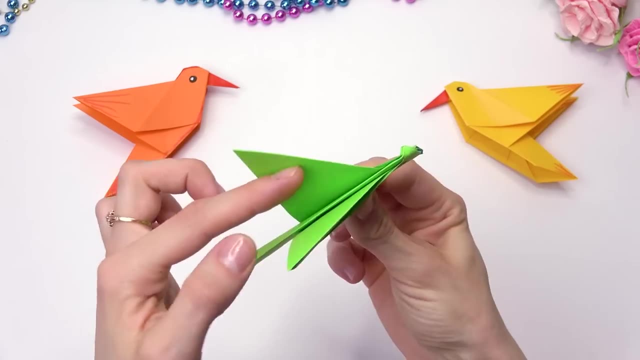 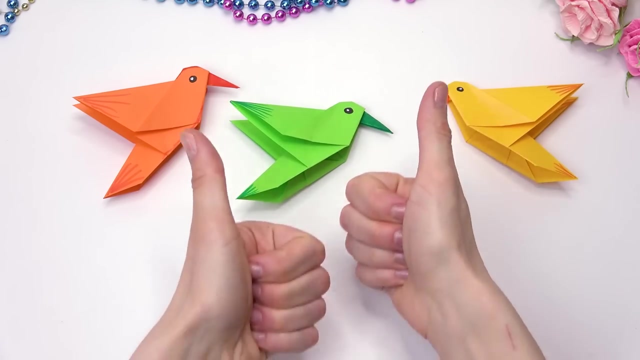 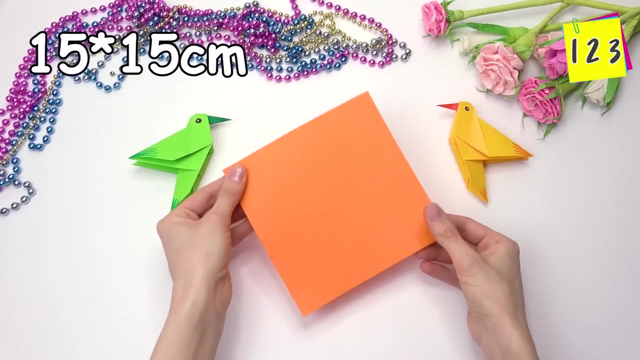 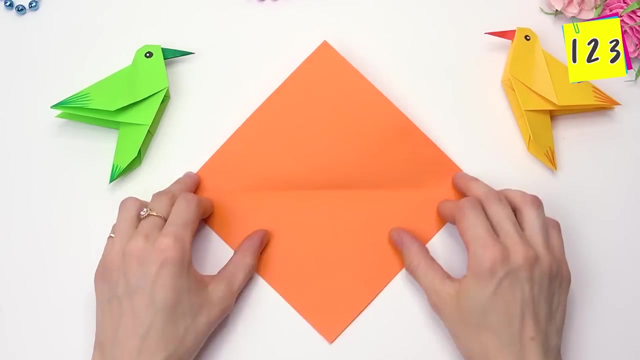 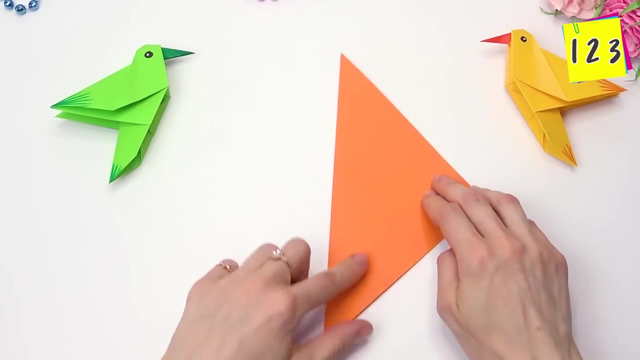 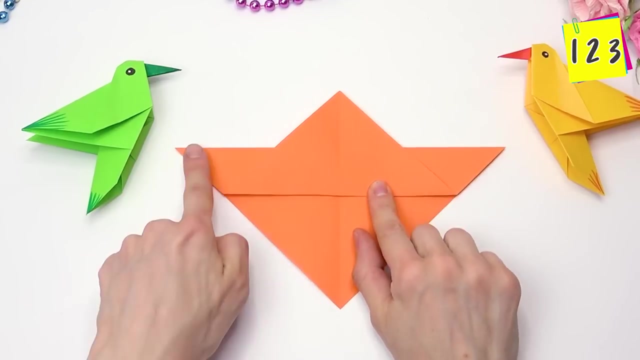 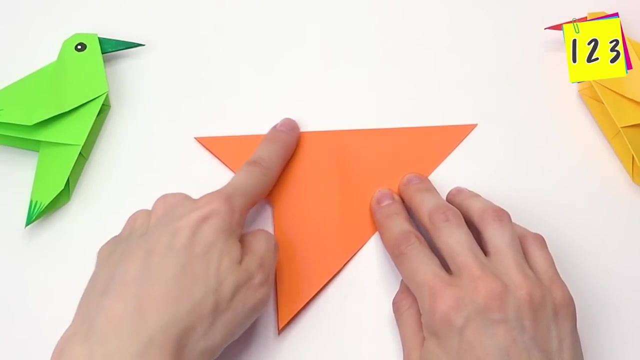 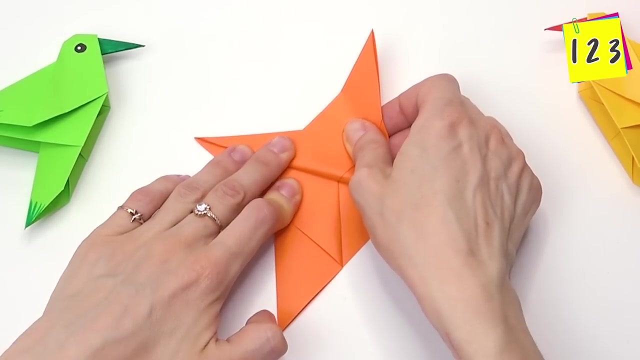 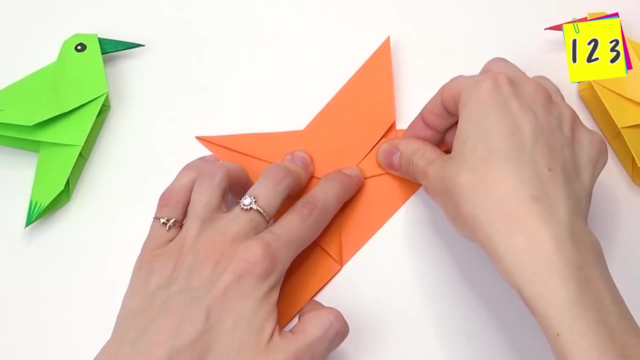 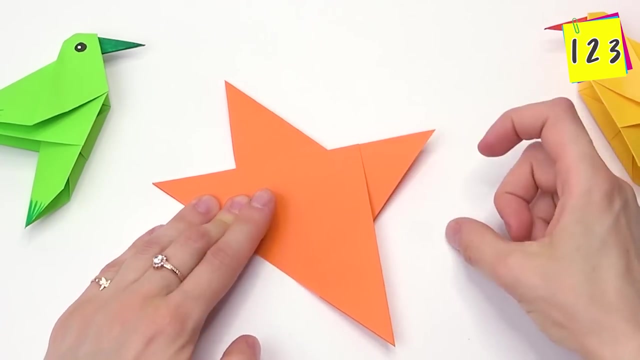 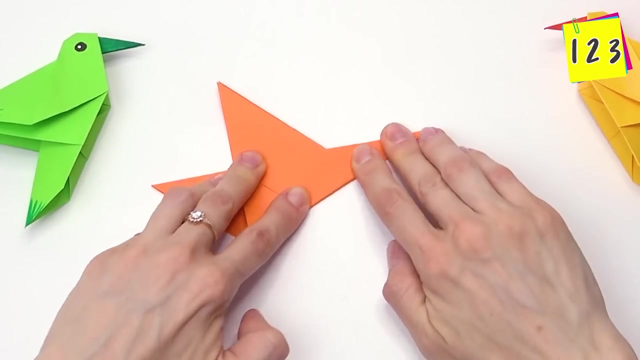 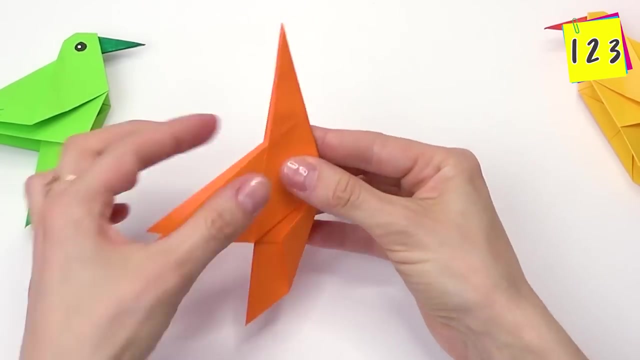 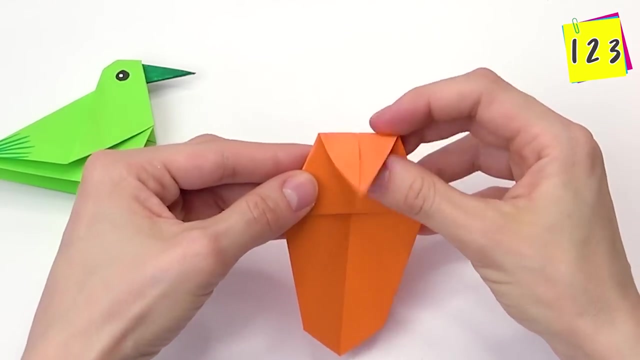 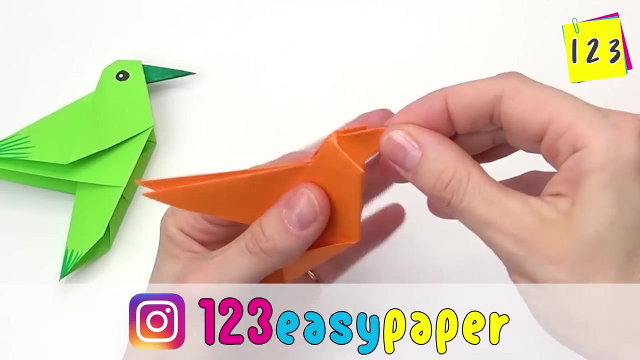 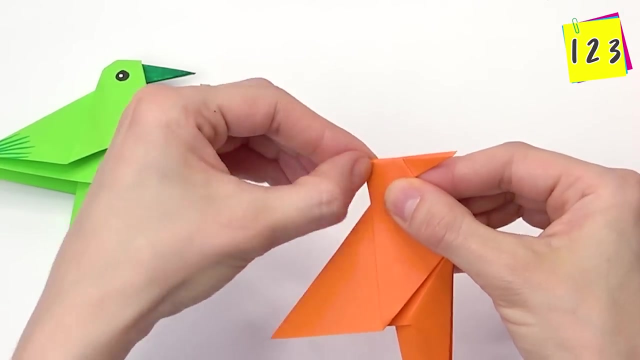 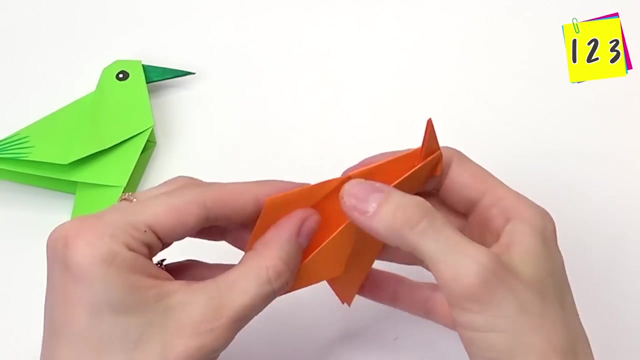 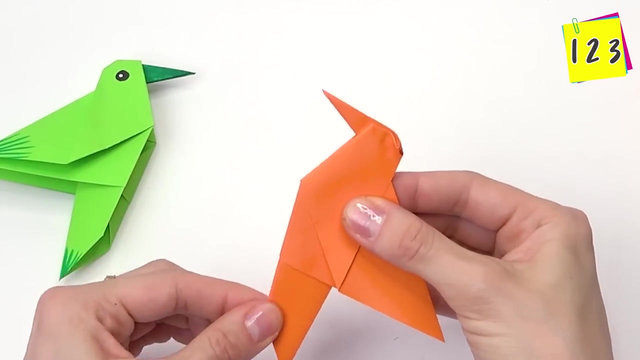 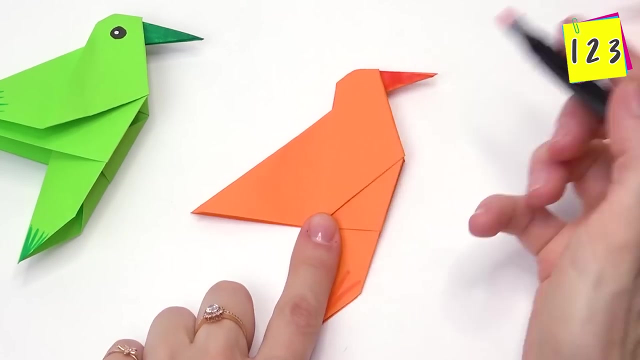 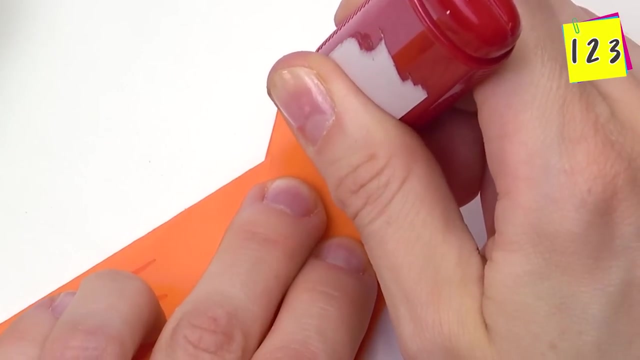 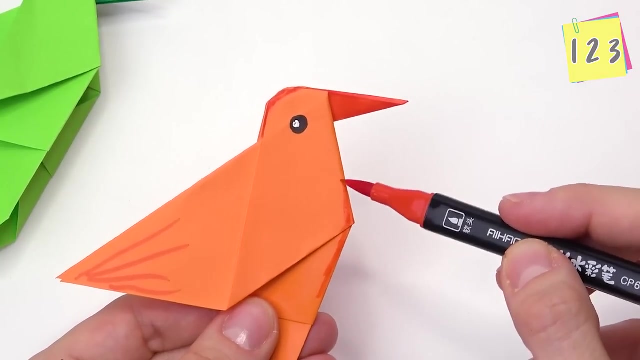